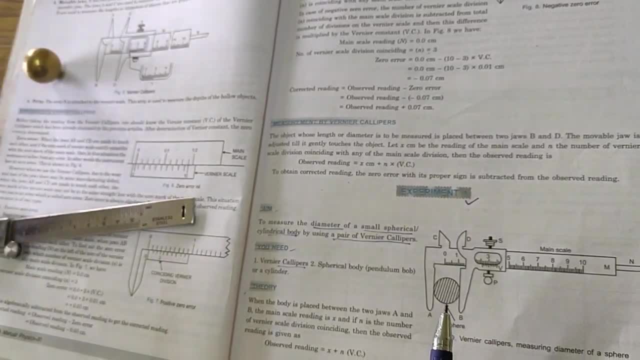 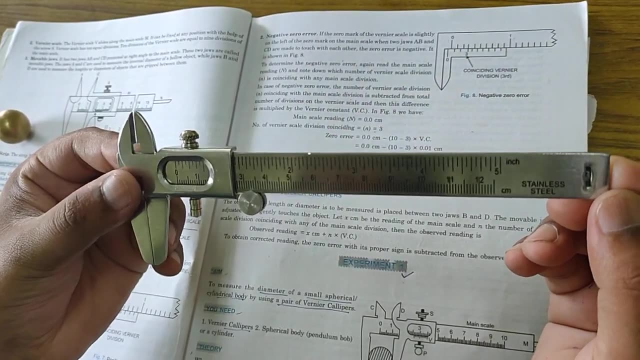 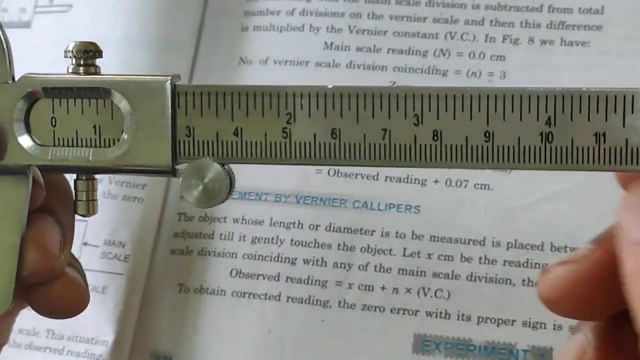 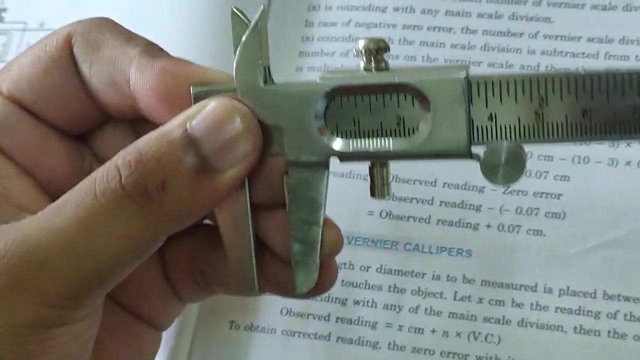 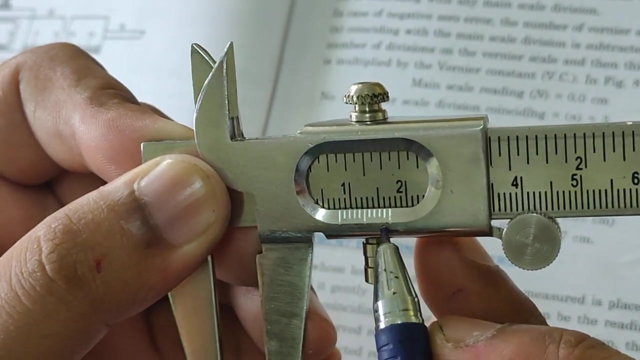 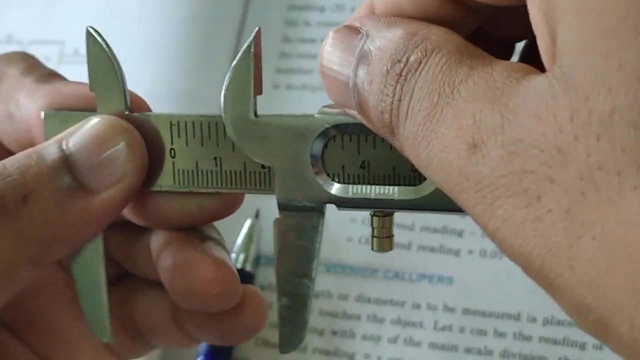 So, before starting, I am going to introduce you the vernier calipers. As you can see, this vernier calipers- see it continues. It contains two scales. First, this one is known as main scale. It is in centimeter as well as in inches, Okay. And the second scale, this, as you can see, this is the vernier scale. Okay, Vernier scale contains 10 division, Okay. And this vernier scale is movable on the main scale Like this: This is the tightening screw. This jaw is known as extension. 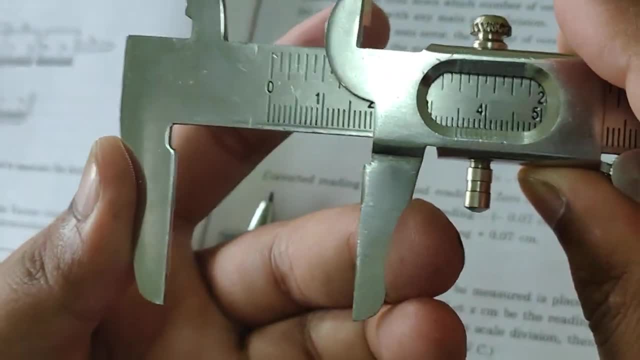 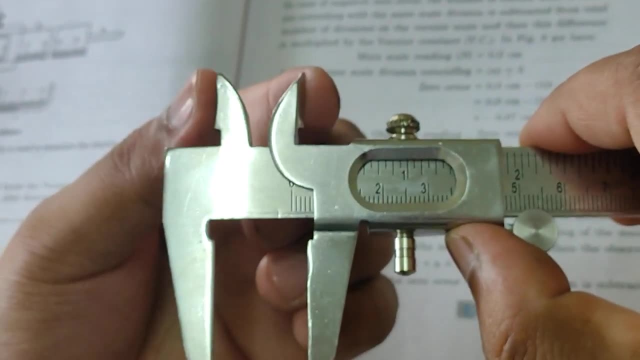 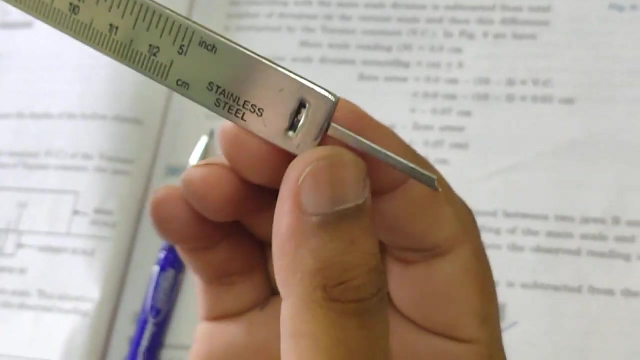 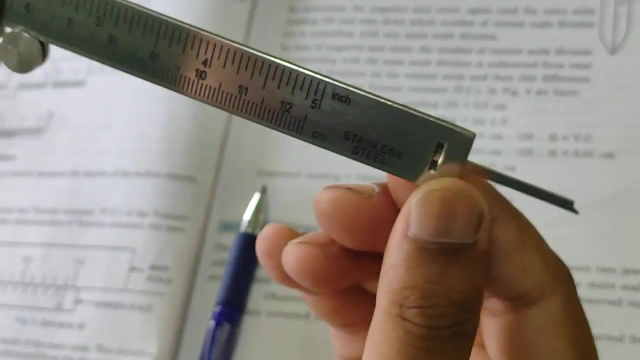 This is the external jaws. By this you can measure the external diameter of a beaker. And these, this jaw, These jaws is known as internal jaws, And by this we can measure the internal diameter of a beaker. And here is another scale. See this, This probe. by this we can use the height of the beaker. As you can see, when this is completely closed and reading is zero. 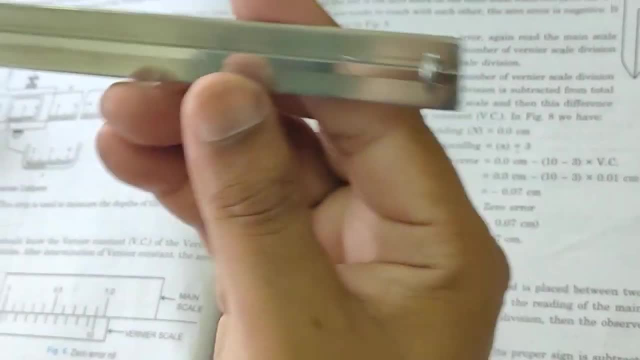 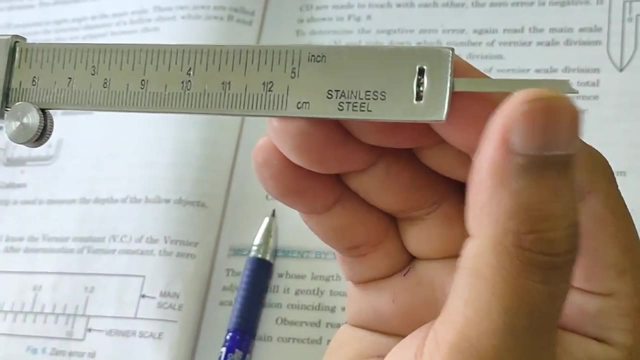 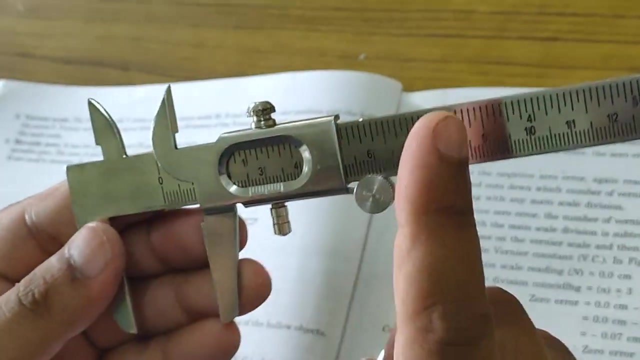 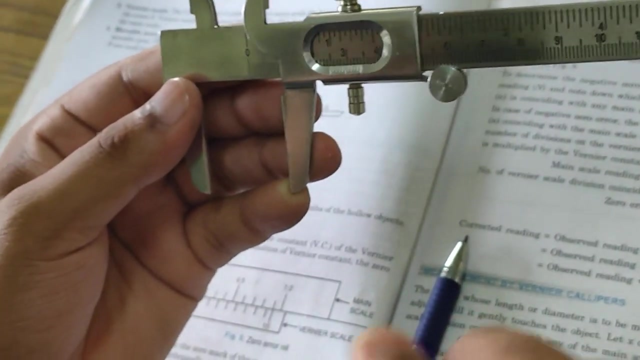 is aligned with the main scale, okay, and as the vernier calipers is moving, so this probe is going to measure the depth. okay, now see. so, as you know that vernier calipers contains two scale: main scale and vernier scale. so first we are going to, we are going to measure the least count of vernier. 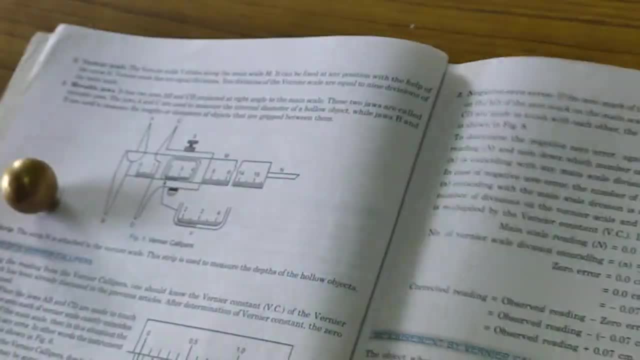 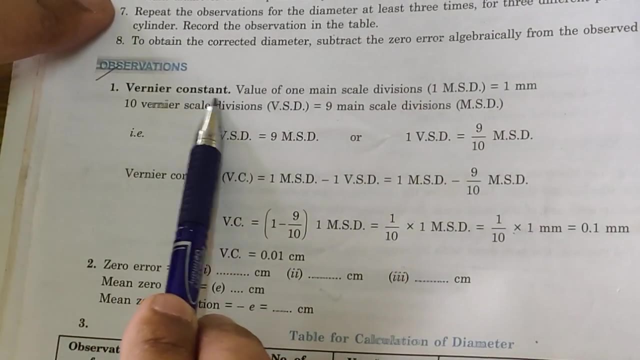 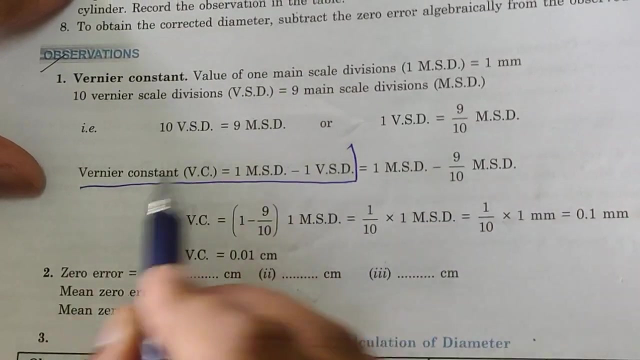 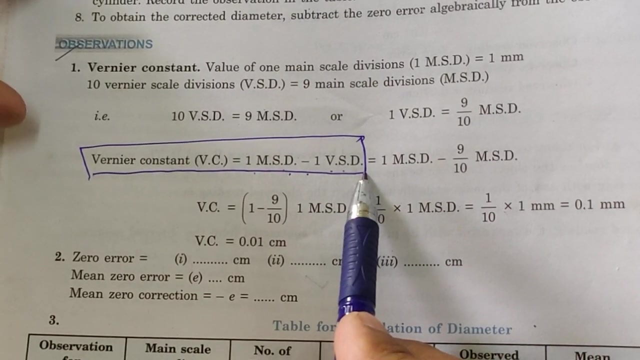 calipers. okay, then see here: the least count of vernier calipers is also known as vernier constant. okay, and the formula for least count of vernier calipers is: this is the very important formula, and that is one main scale division minus one vernier scale division. okay, now see, since we 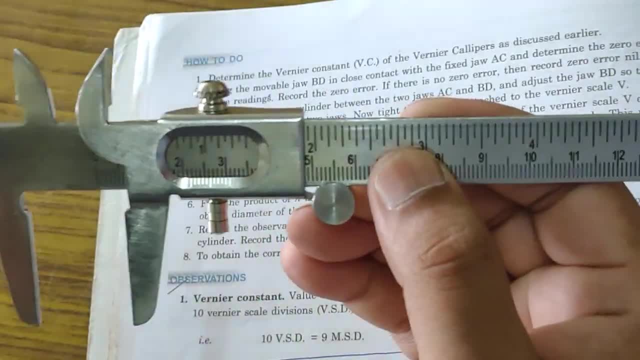 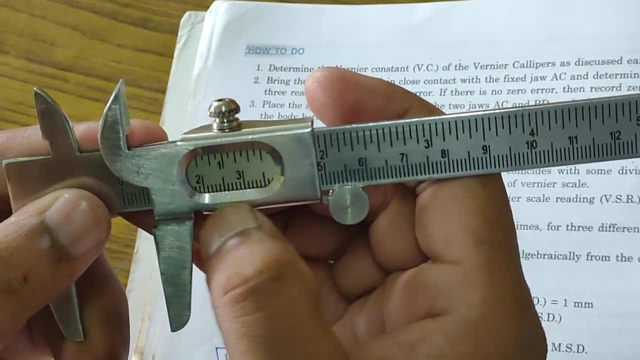 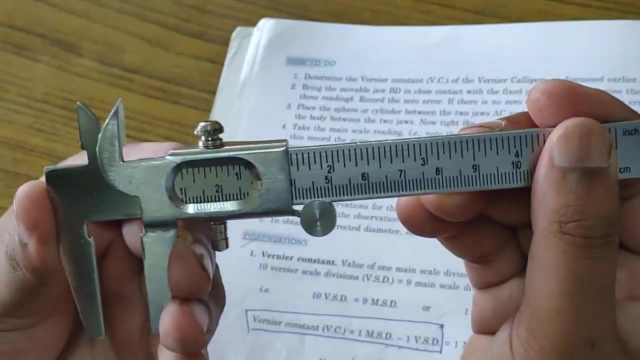 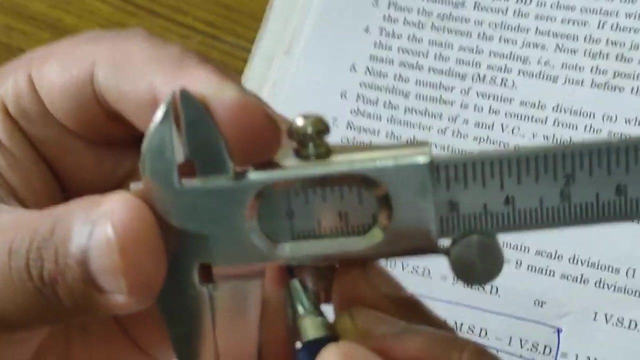 know that. see here in, see here in. since we know that we have unit only in main scale. vernier scale has no unit. so we have to convert this vernier scale into main scale. okay, and how we are going to do it. see first, close the jaws and, as you can see, this zero mark of vernier scale, this zero mark of vernier scale, is aligned. 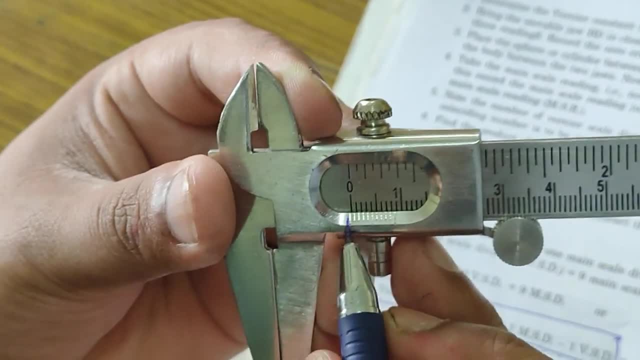 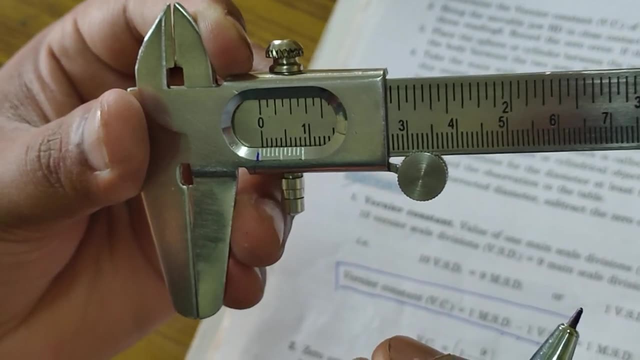 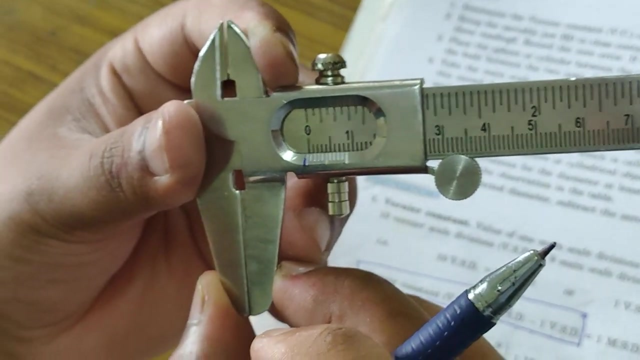 with the zero mark of main scale get. that means this particular instrument has no error. we are also going to discuss negative and positive error, but that is in second video. see. so this 0 when aligned with the main scale 0, the instrument has no error and, as you can, 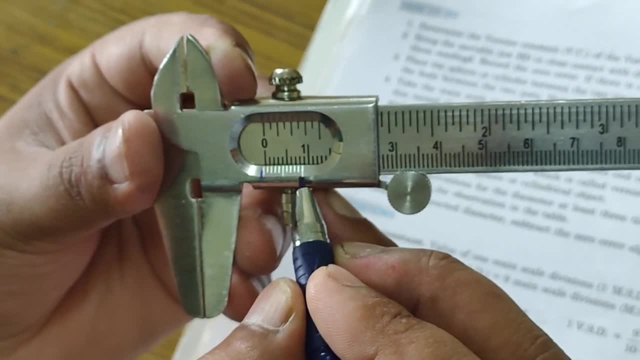 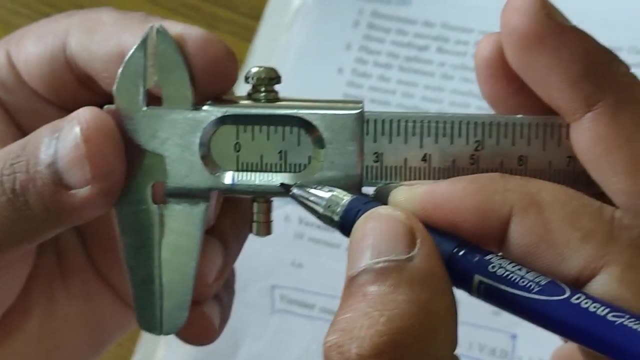 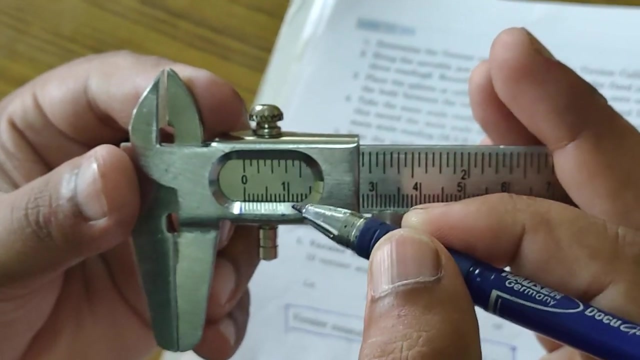 see the 10 division of vernier scale match with the 9 division of main scale. see very carefully. the tenth division of vernier calipers. this one match with the ninth division of main scale. okay, so we can write here. see. see, since the tenth ten division of. 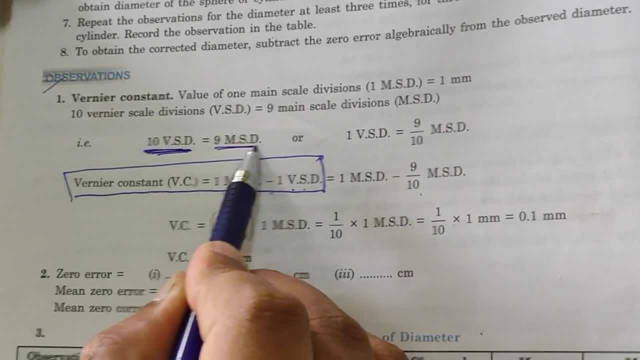 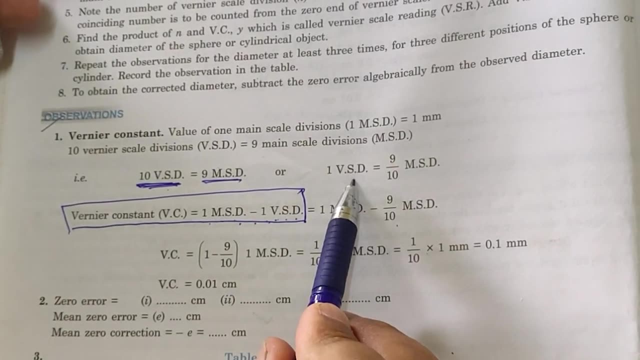 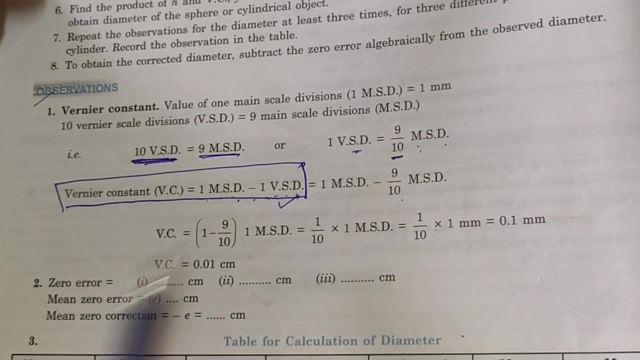 vernier scale is equal to nine division of main scale. so we have to find out the value of one vernier scale division. so from here we can find out the value of one vernier scale division, and that is equal to nine by ten main scale division. we are placing this value over here so this become 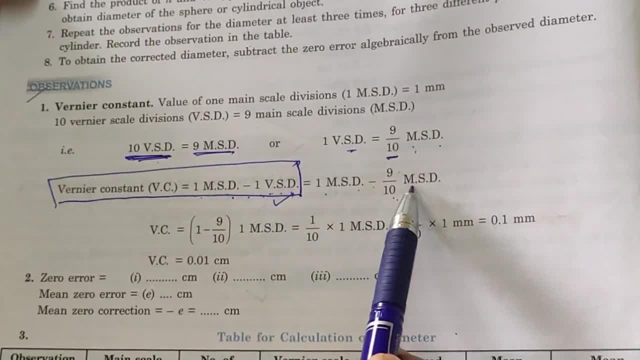 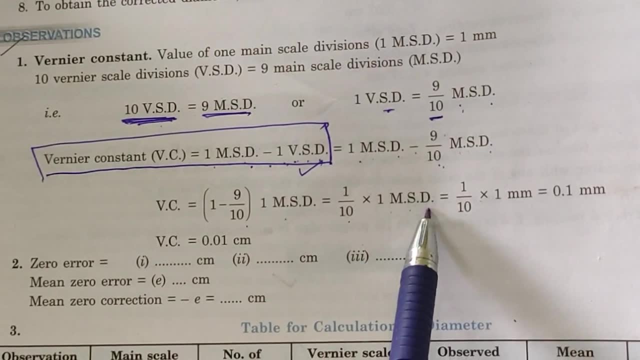 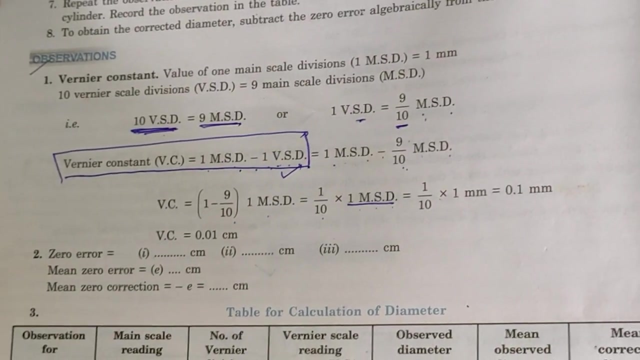 one main scale division minus nine by ten main scale division and on subtracting this, we have one by ten of one main scale division. okay, now what we have to find out the value of one main scale division in which the unit is contained. okay, now, as you can see the main scale, or you can see 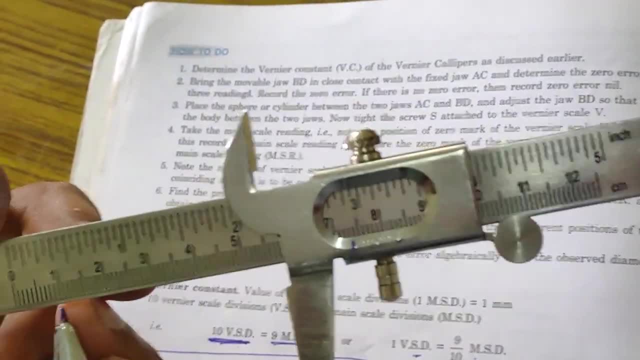 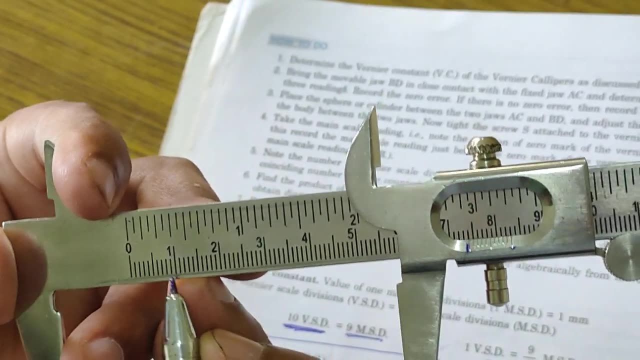 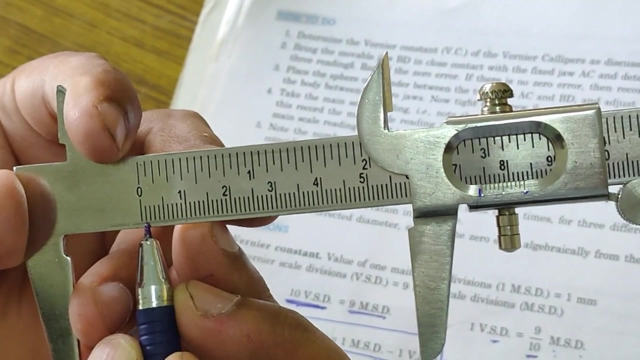 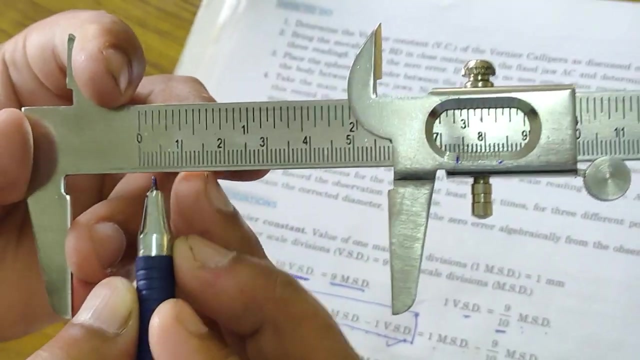 there the least count of main scale. this main scale is simply your centimeter scale, so, as you can see, one centimeter centimeter is divided into 10 division. so the value of one division is simply 1 by 10 centimeter, or 0.1 centimeter or 1 mm. okay, this is also known as least count of main scale. okay, least count of. 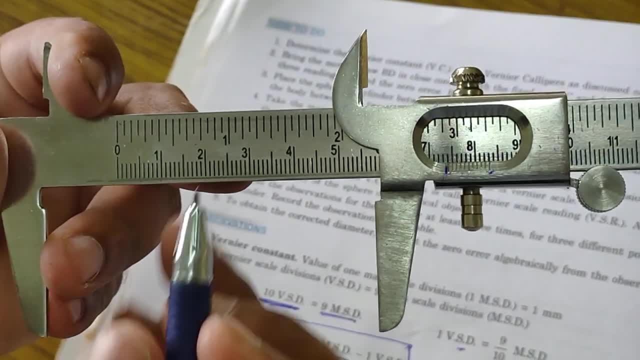 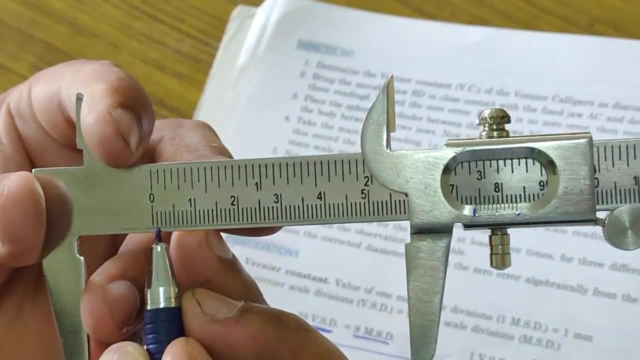 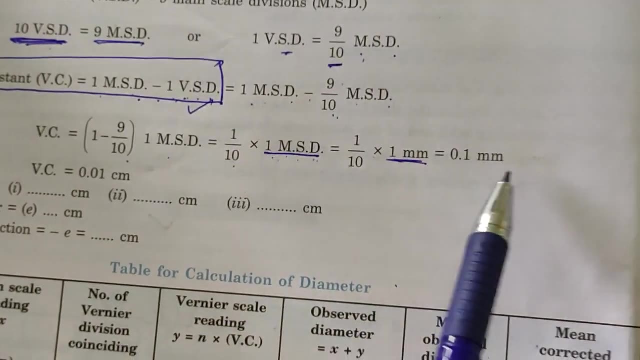 main scale, not the least count of vernier calipers. so see so 1 msd, one main scale division, is equal to 1 by 10 centimeter or 1 mm. so see here, 1 msd can be replaced by 1 mm. so 1 multiply by 1 by 10. 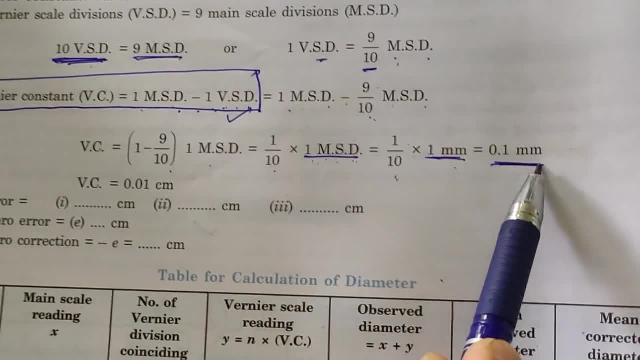 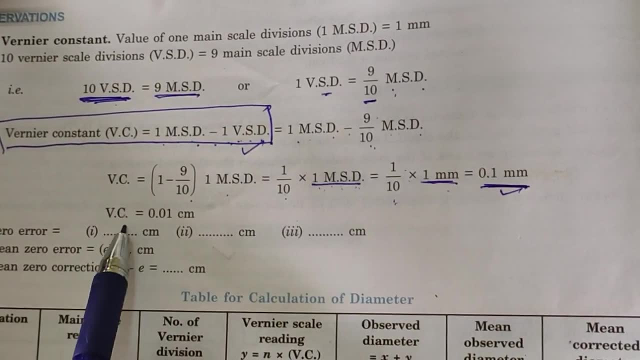 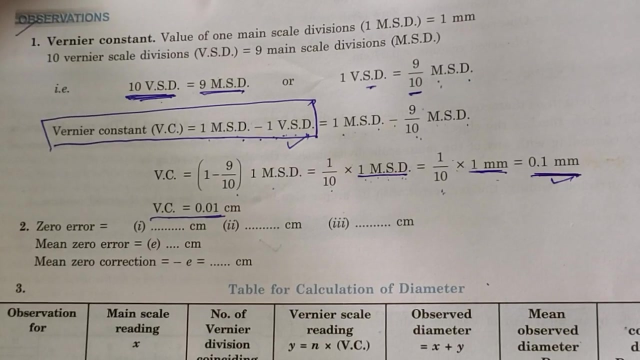 mm, so it simply becomes 0.1 mm. so this is the least count of vernier calipers, or this is also known as vernier constant, in centimeter. we can write this: vernier constant is equal to 0.01 centimeter. as well as you can see this particular instrument. 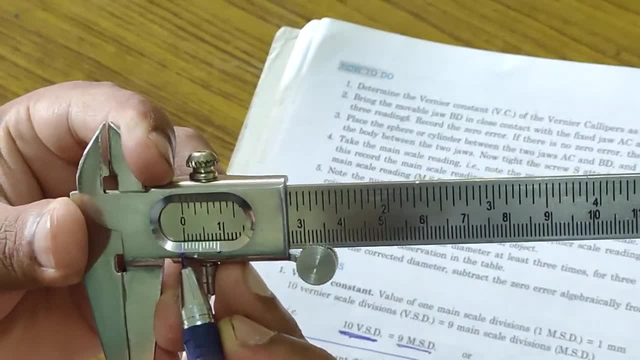 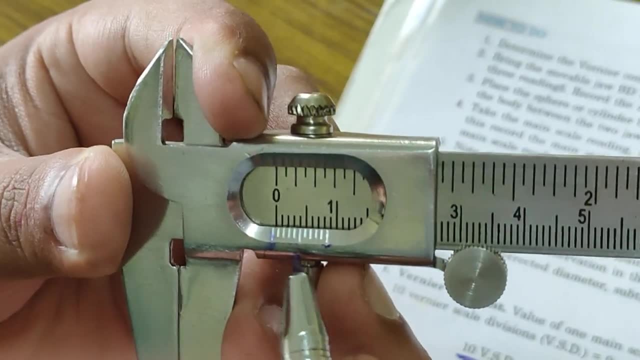 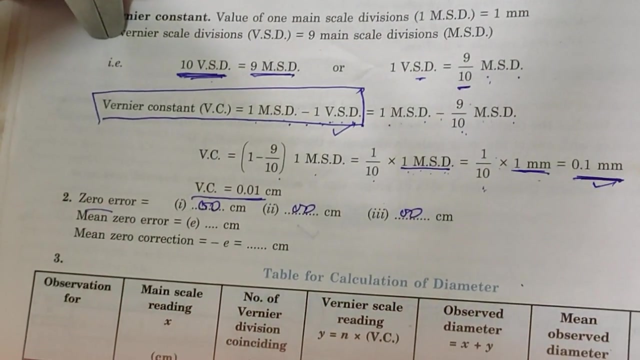 zero division of vernier scale coincide with the zero division of main scale. that's why this particular instrument has no error. so in the column of zero error it's simply zero centimeter. okay for the whole reading, and that's why it is also zero. so no positive. and. 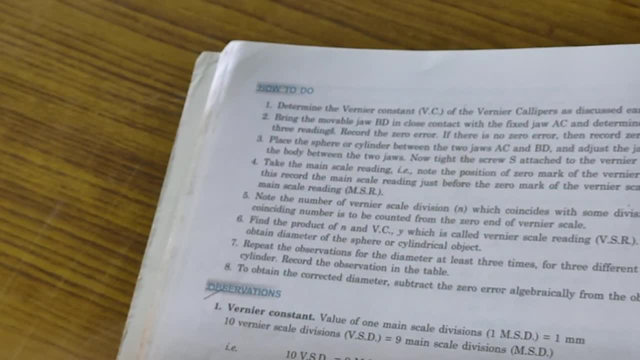 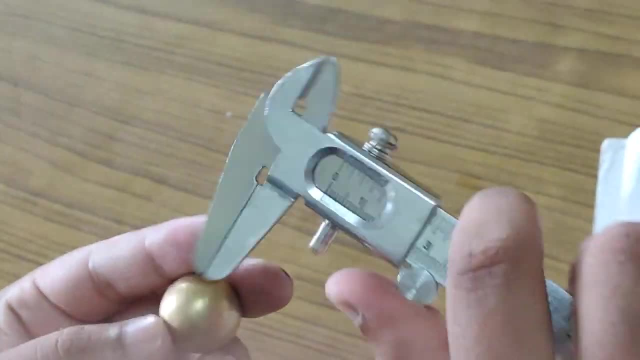 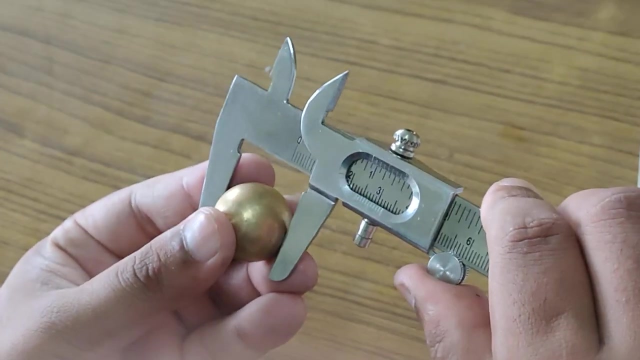 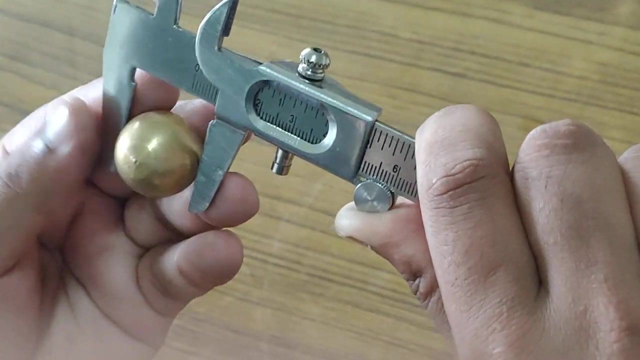 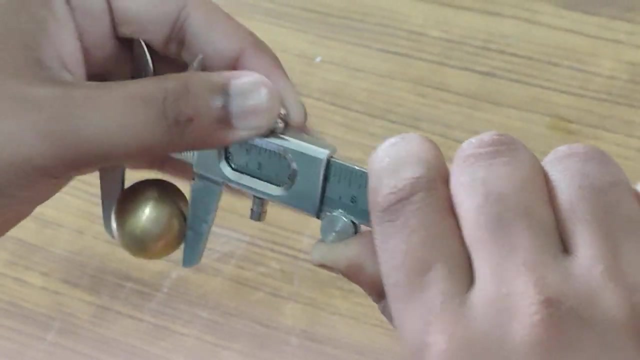 negative error applied here, then now we are going to see how to solve this problem. so now we are going to measure the diameter of the ball. now see, simply take the ball, expand it like this and hold it like this. after this, you have to tighten this screw so that, if the body is suddenly 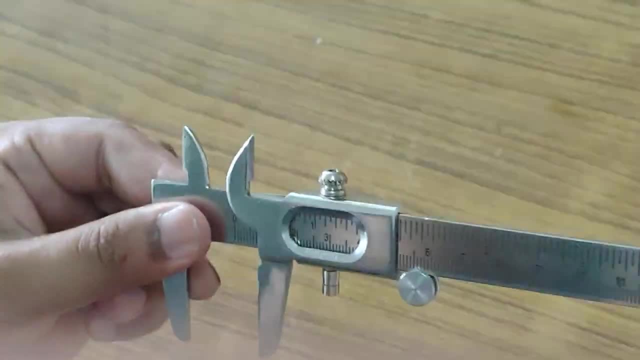 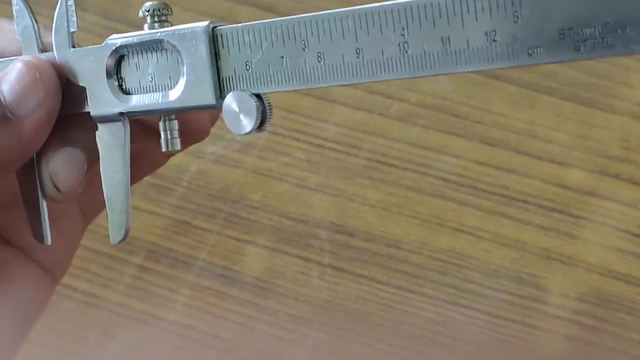 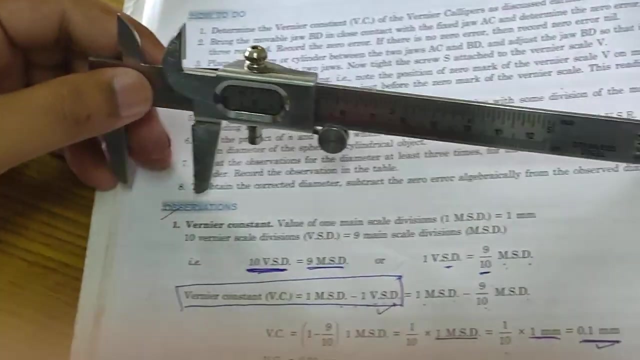 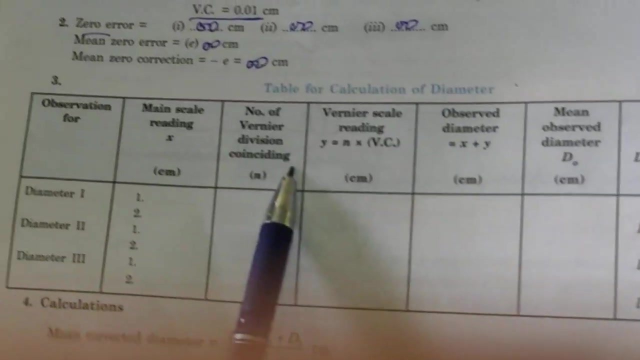 removed like this, so your building do not disturb. okay, now we are going to take the reading. now see the reading. the reading table is looks like this. see very carefully. this one is the first. diameter reading. okay, main scale reading: the number of vernier division that concise with the main scale, then vernier scale reading, then total reading. that is mixed up then. 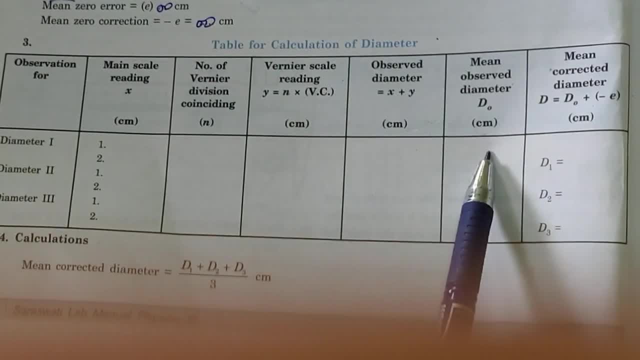 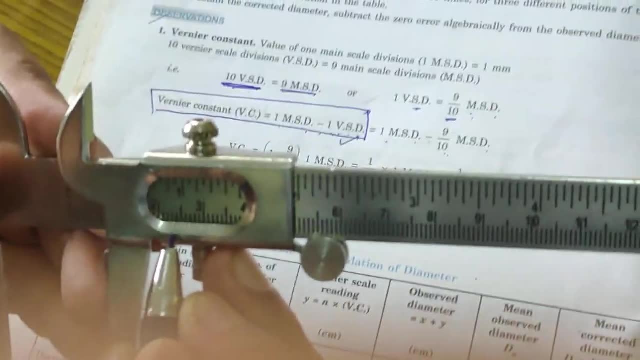 it is moving at an automatism. then will be the table one. this is the table, another one is met skyscrapers, then one and then mean diameter. Now see what is the value of main scale reading. Main scale reading is the reading, the total reading, which is already covered by the vernier scale and to the left of the vernier 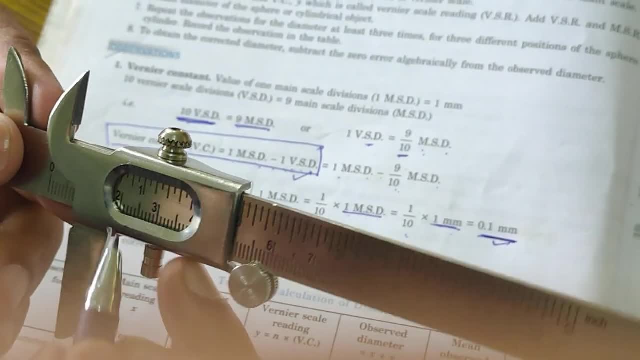 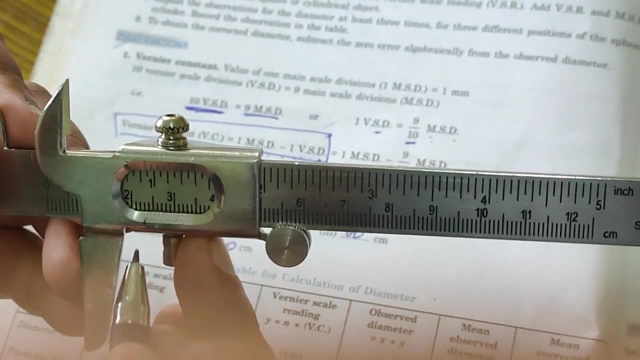 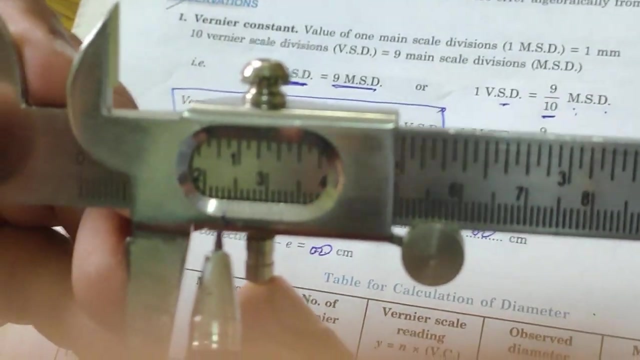 scale Now. as you can see, this 0 mark is lies between 2.3 and 2.4.. So it is between 2.3 and 2.4.. 2.3 is already completed, Sir. please zoom karengi thoda. sir, Now see very carefully. 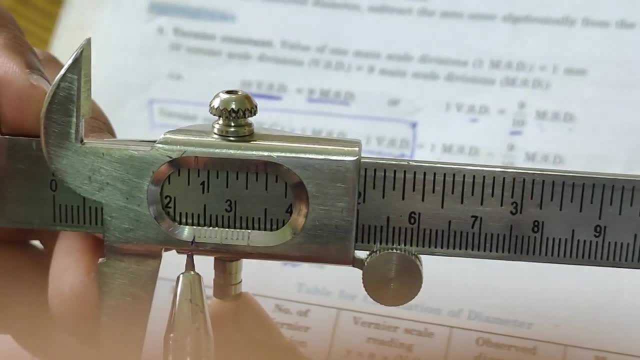 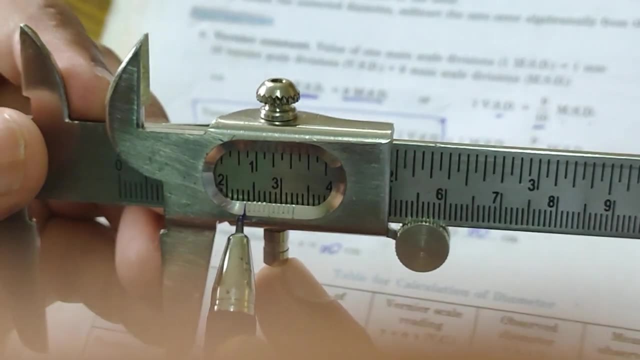 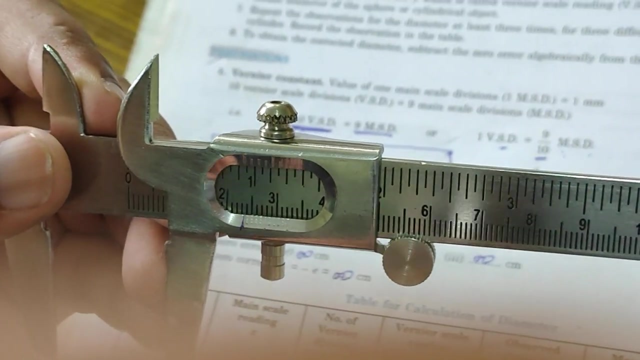 to this: 0 mark is exactly lie between this is 2.3 and 2.4.. So 2.3 is completed and 2.4 is not. So you can say that the diameter of spherical bob should be lies between 2.40. 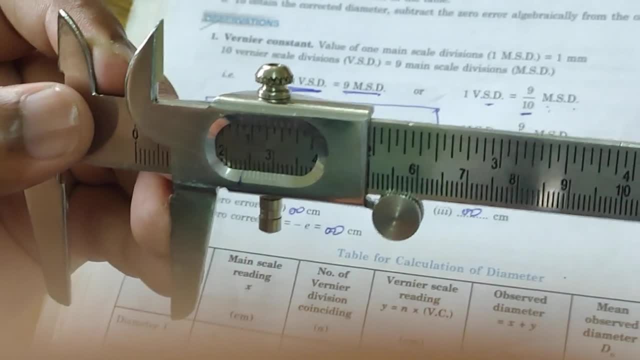 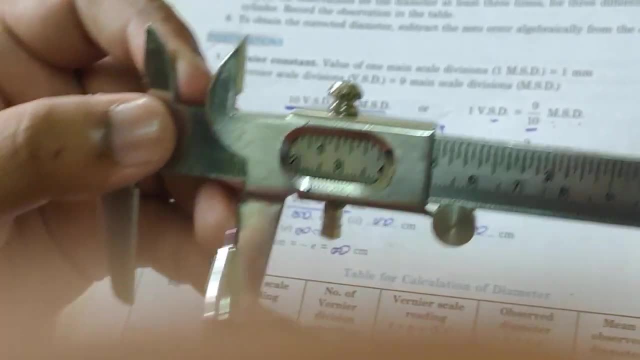 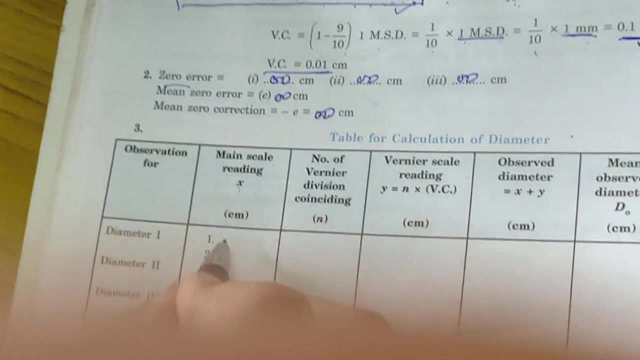 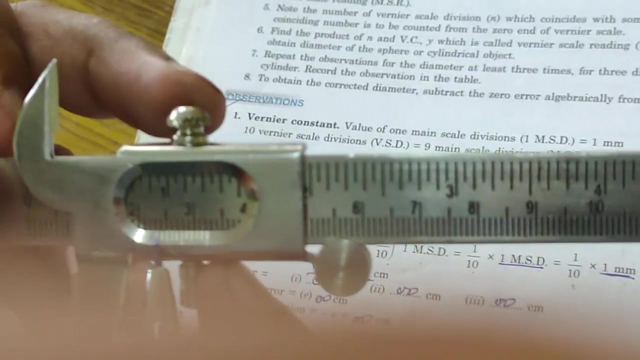 and 2 point sorry, 2.30 and 2.40. okay, Now see. so 2.3 is completed. so complete reading is reading of main scale. So see here reading of main scale which is completed, or the reading which is left towards the vernier scale. So it is 2.3 in centimeter. okay, Now see this first division is: 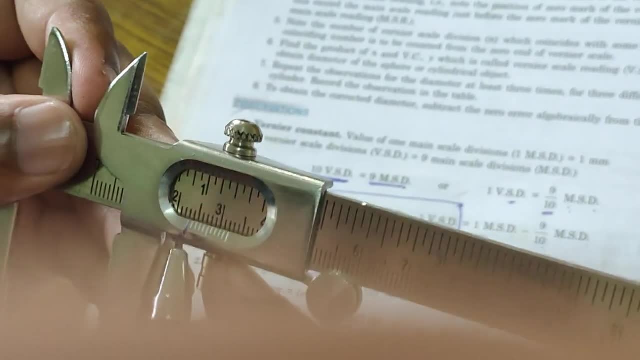 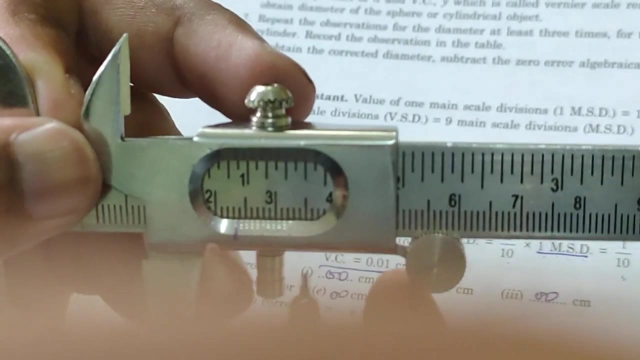 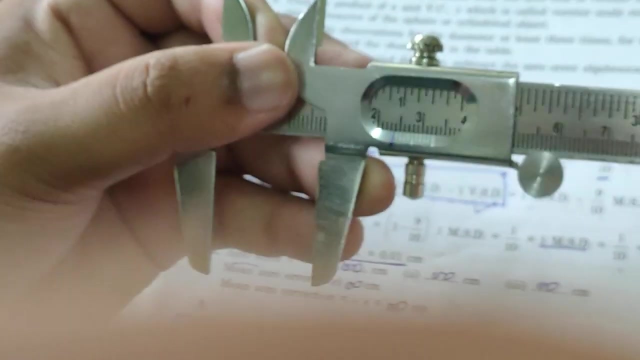 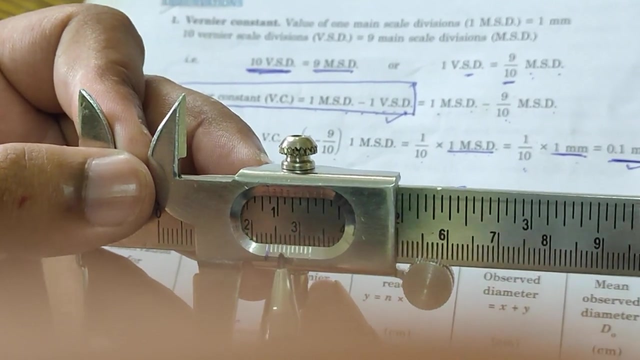 0 and it is not coinciding with the main scale because it is lies between 2.3 and 2.4.. Now you have to find out what division of vernier scale exactly coincide with the main scale. okay, So, as I can see very carefully, see 0,, 1,, 2,, 3, 4, this fifth division, This fifth division coincide. 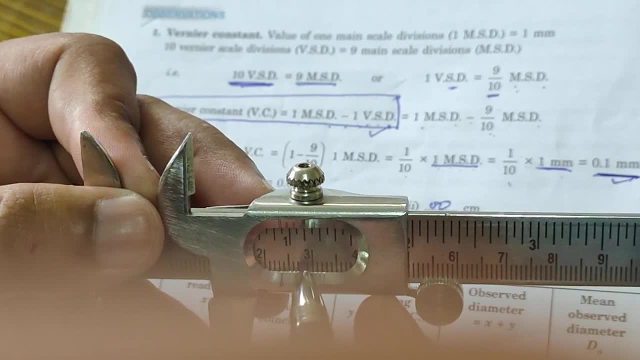 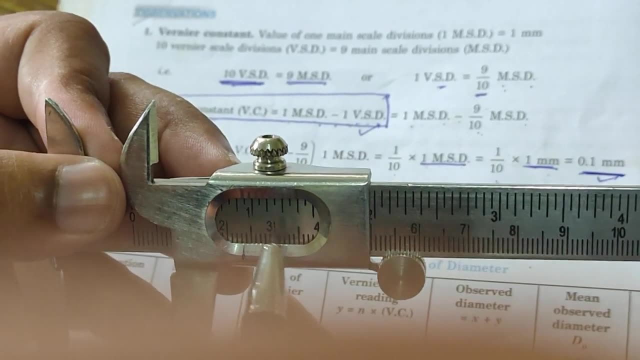 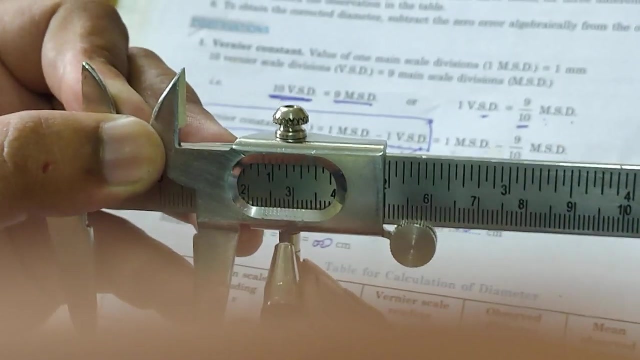 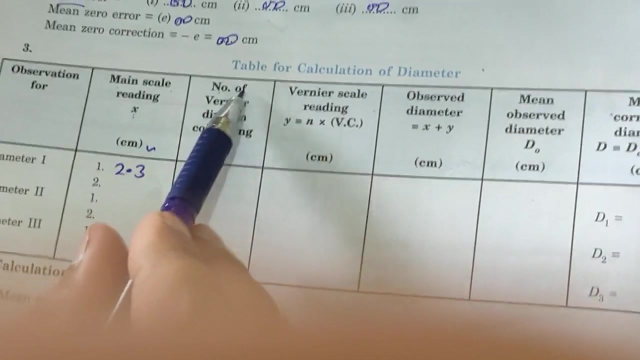 exactly with the 0.. 1 of the division of main scale. okay, So you have to just see what division is exactly coincide with the any of the division of main scale. So in this case, fifth division is: coincide with, exactly with the main scale. So n, this small n, that is number of vernier division coinciding. 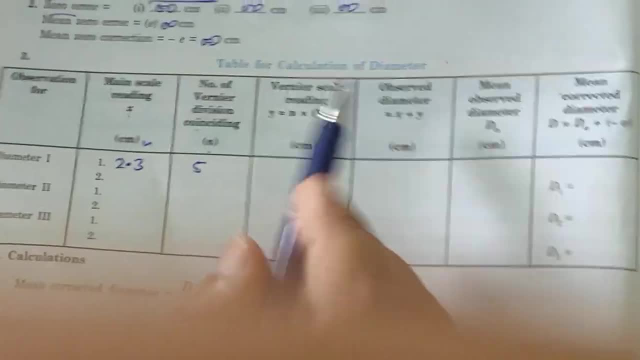 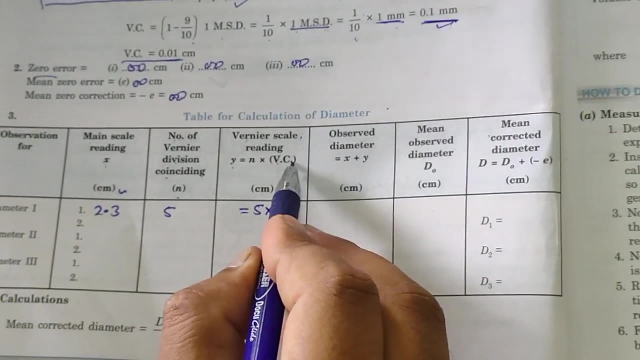 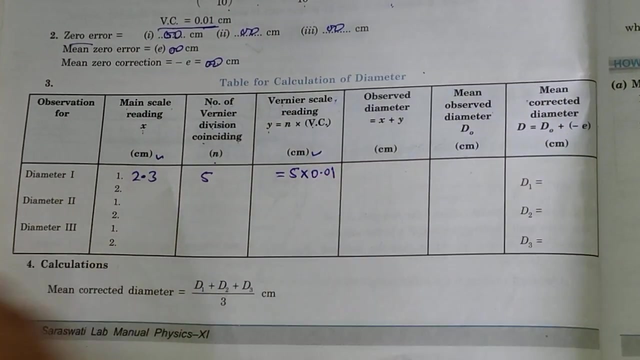 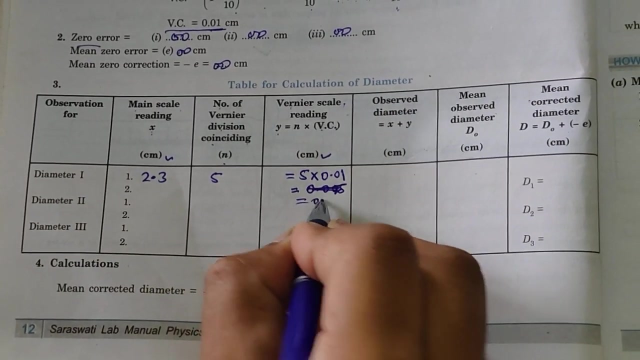 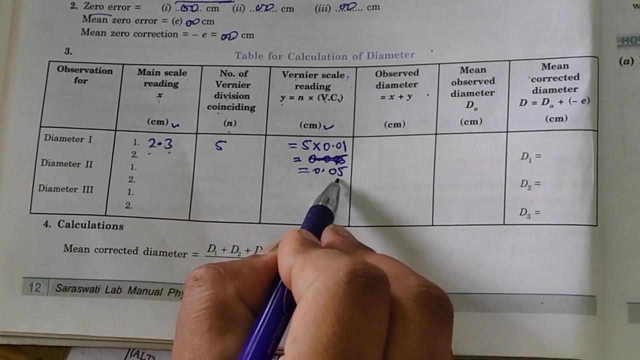 is 5. okay, Now see vernier scale reading. that is simply 5 into vernier constant and that is least count of vernier calipers. So it is 0.01 in centimeter. So it looks like 0.05. sorry, 0.05, okay. So the total observed reading become 2.3 plus 0.05.. So it become 2.35.. 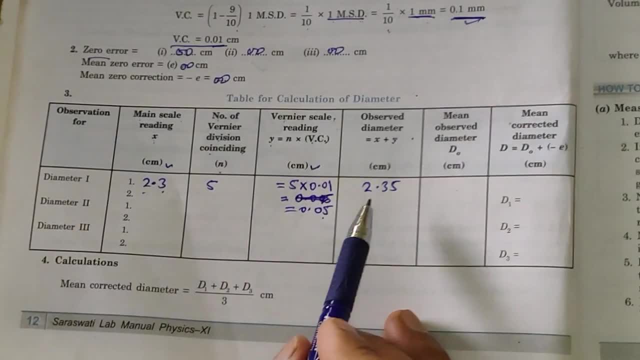 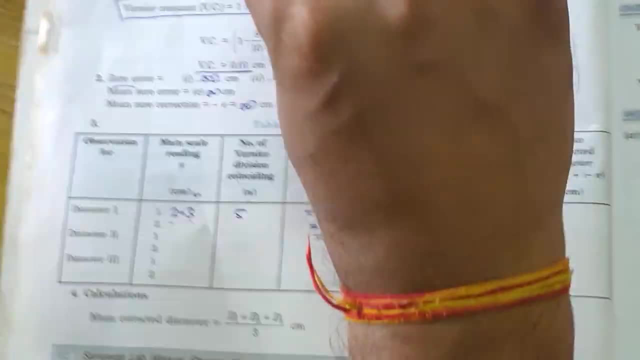 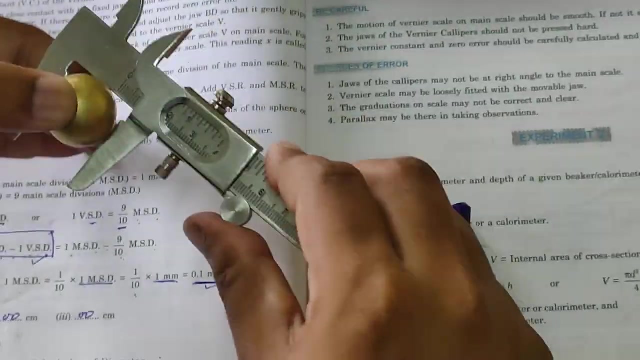 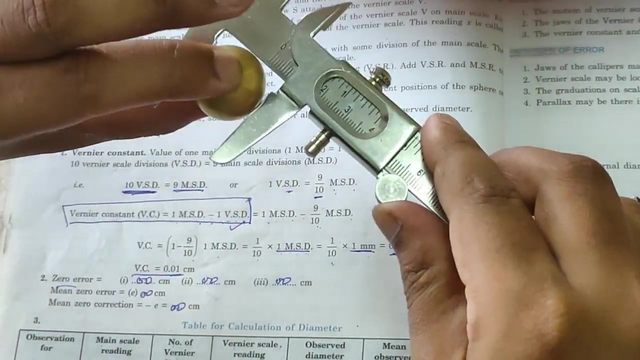 So, as I told you, the eject reading is between 2.30 and 2.40. ok, So this is your first diameter. ok, now for the second reading. see now. see. in the first we taken the reading like this: see, there is a hole in a spherical bob here. I hold it like this and reading of this spherical 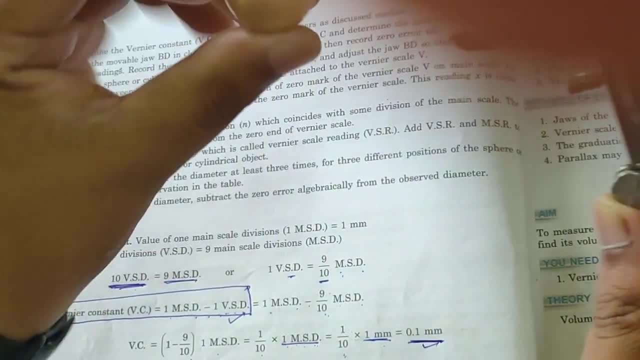 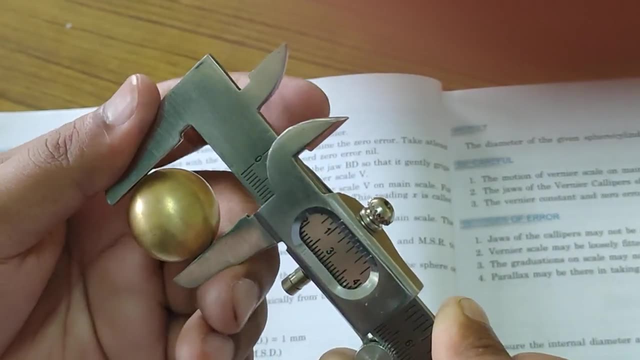 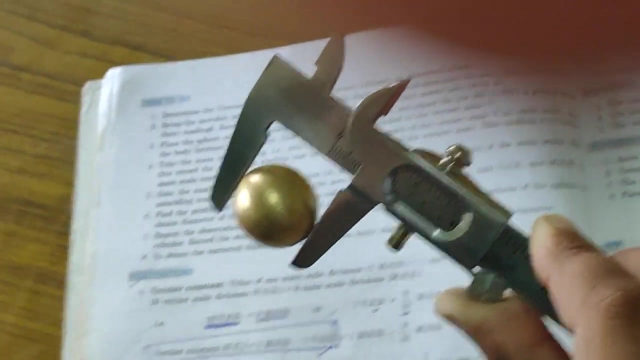 bob is like this: ok, in the first case. In the second case you have to take this like this: ok, perpendicular- ok. So in this case, reading is like this: ok, because, since this is spherical bob, sometimes if the spherical bob is not uniform, it not necessary that two. 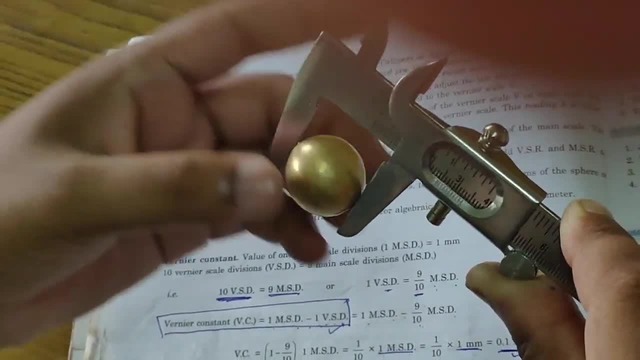 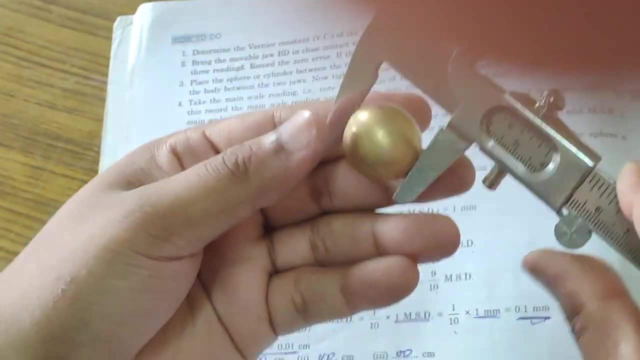 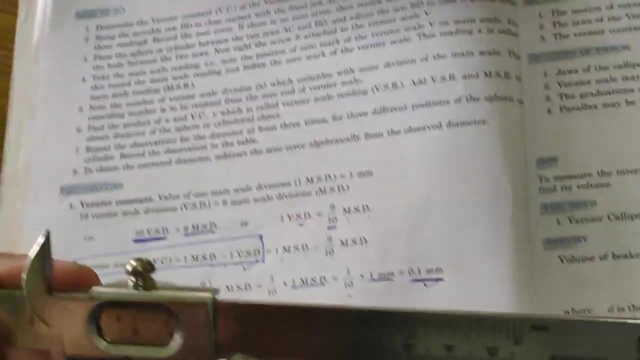 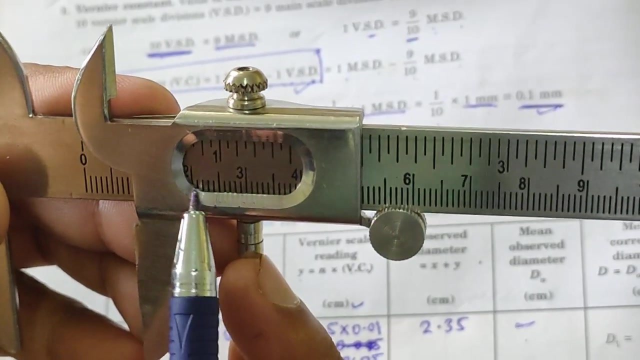 readings becomes same or comes out to be same, ok, So in this case, see, we hold it like this and tightening this screw, ok, and we can remove this. Now see very carefully, see, in this particular case, reading get changed. in this case, see, this zero of vernier calipers lies between 2.4 and 2.5.. So I am going to measure it. 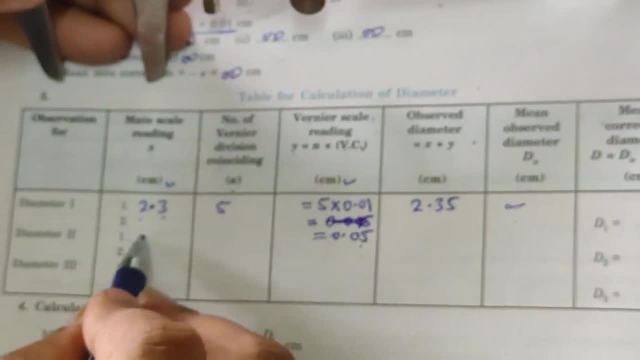 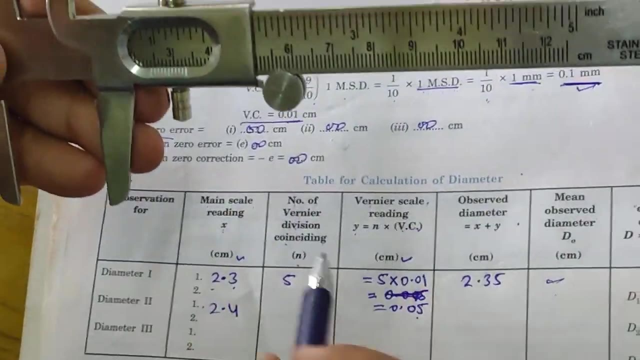 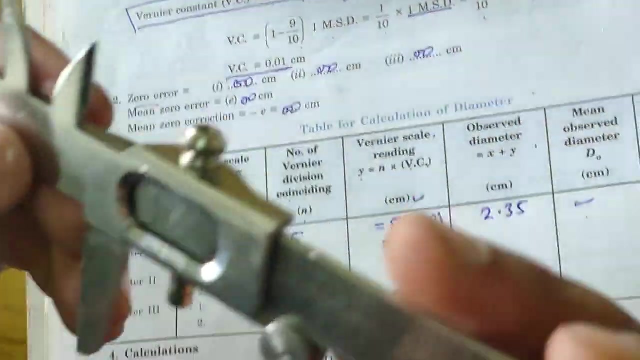 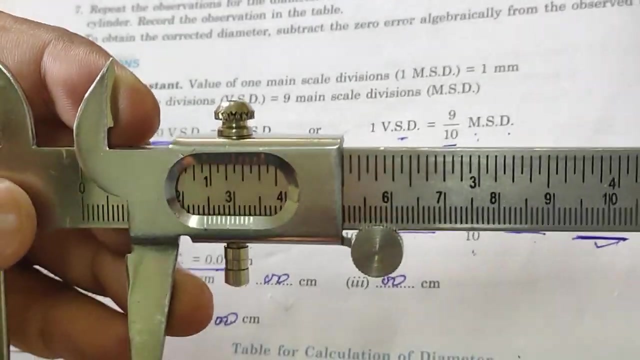 so again see this diameter. second, the main scale reading is 2.4, since it is left to the zero division of vernier scale. ok, Now see for number of division which coincide with the main scale. see, so, as I can see, one second, So as you can see. so please zoom it as you. 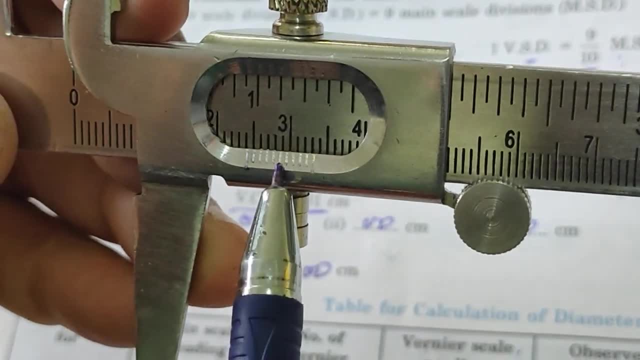 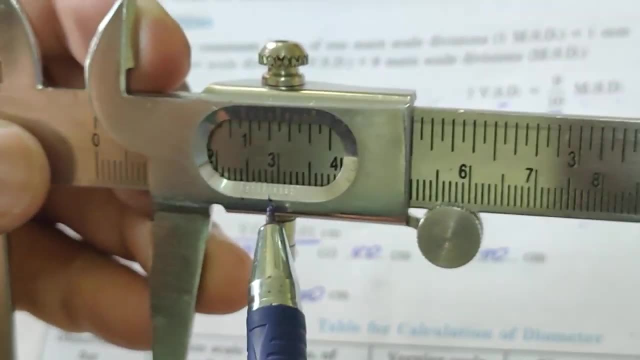 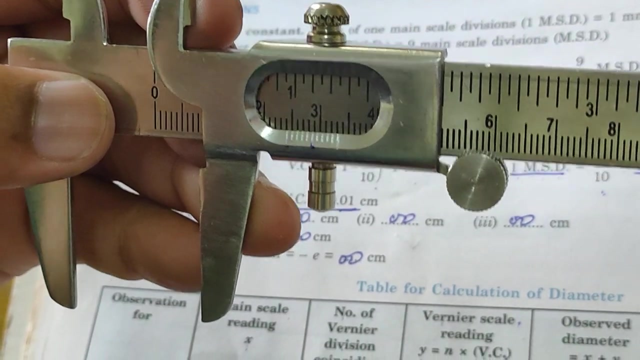 can see. in this case also, this fifth division is coincide with any one of the division of main scale. this fifth one, ok. One more thing: different student can see different division. So, as I can see, the fifth division is coincide with the main scale. ok, It is just for practical. 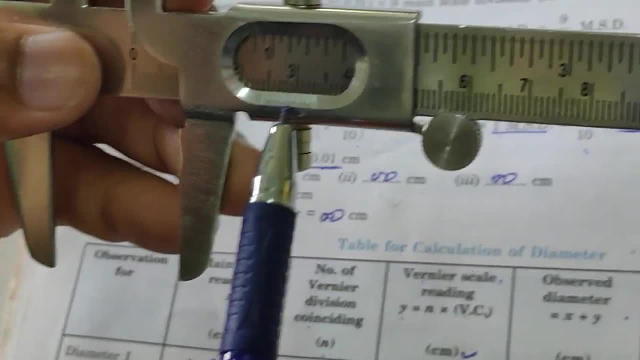 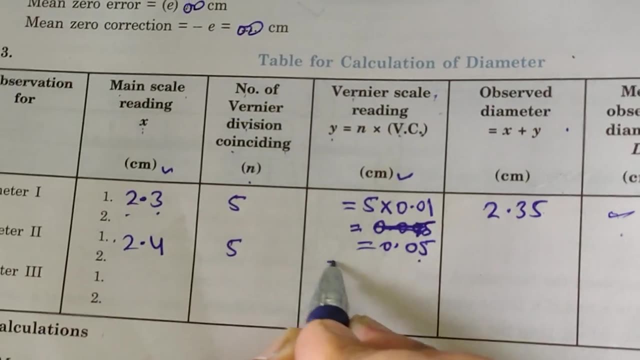 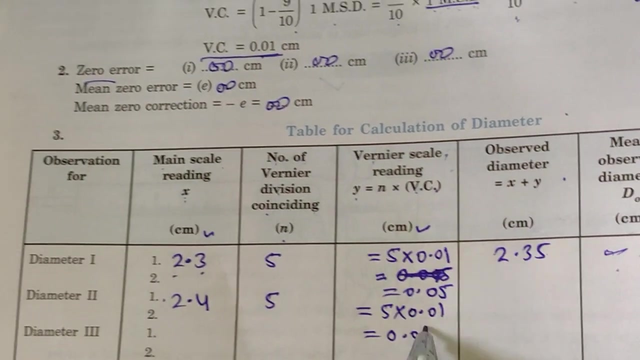 purpose. ok. So the, let us say, 5.. So, as I can see, fifth division is coincide with the main scale. so again, reading becomes vernier scale. reading is 5 into 0.01, that is vernier constant, So it is 0.05. on adding reading become 2.45 in centimeter. ok. Similarly you. 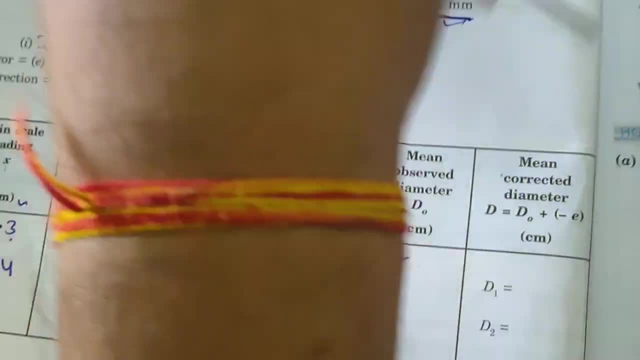 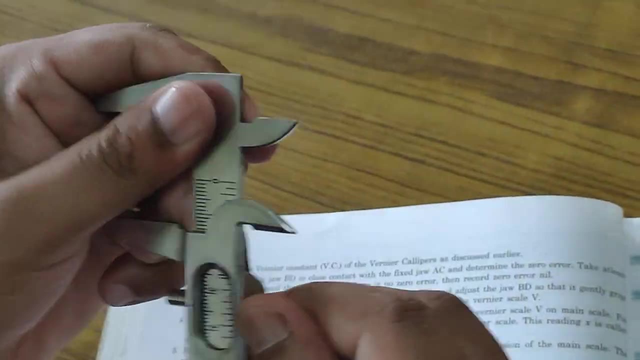 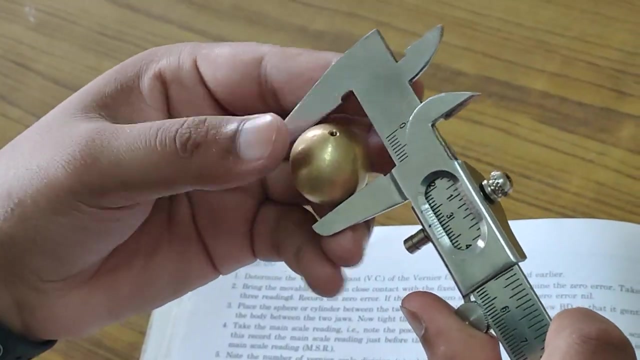 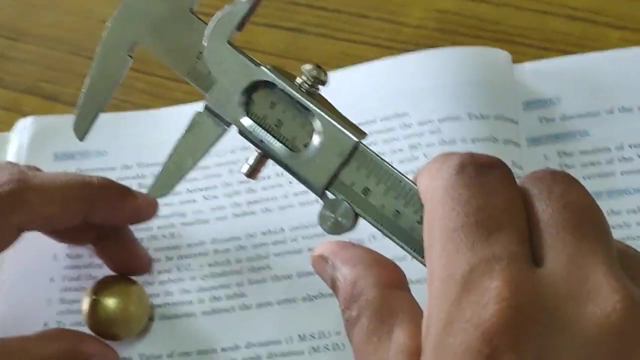 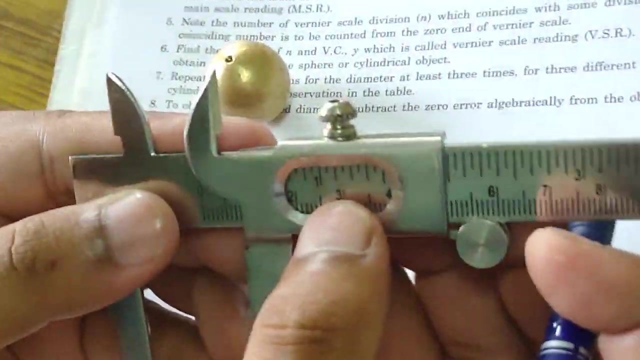 can take third reading also. okay, for third reading, you can. you can take any random orientation of this spherical bob, any random orientation at this spherical bob. okay, so this is a random orientation, tightening the screw and you can calculate the reading again. so, as you can see in this particular case, see this is very important case. third one: see in this particular 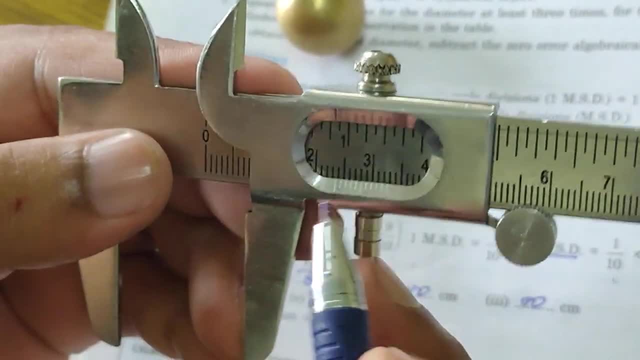 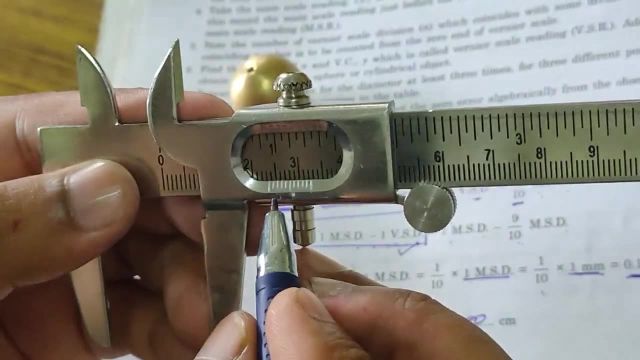 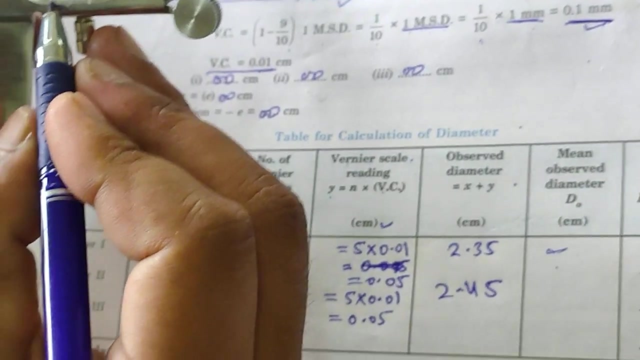 case. you can see the zero division is exactly coincide with the main scale division. so sometimes if that happen, see very carefully: two point four. two point four is already completed. so main scale reading is two point four and zero division is coincide with the two that main scale division. 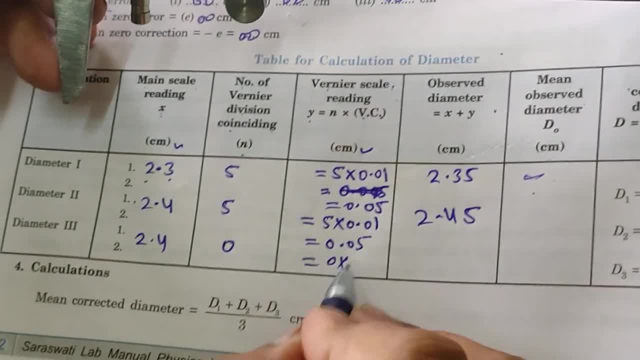 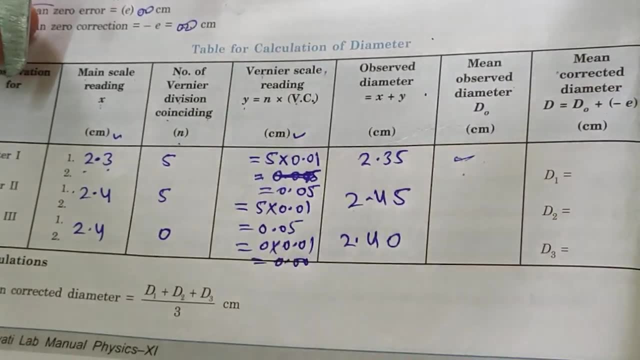 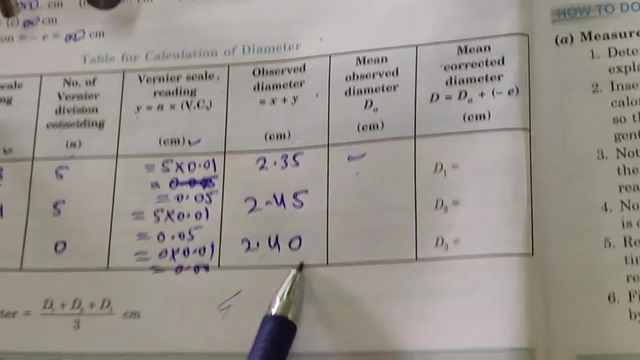 So here is zero and simply zero into zero point zero one. so the one year scale reading become zero point double zero. so the total reading become two point four zero. so, as you can see, one year scale can measure the digit up to two points after the decimal. okay, so, 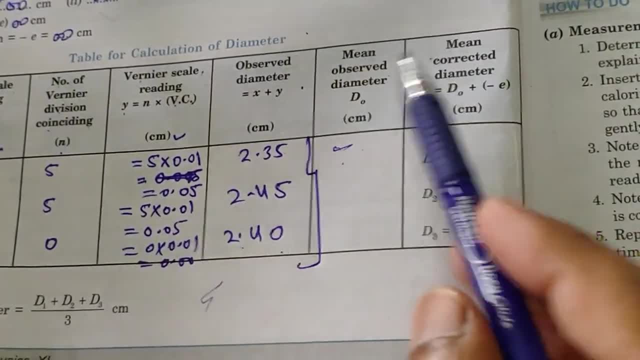 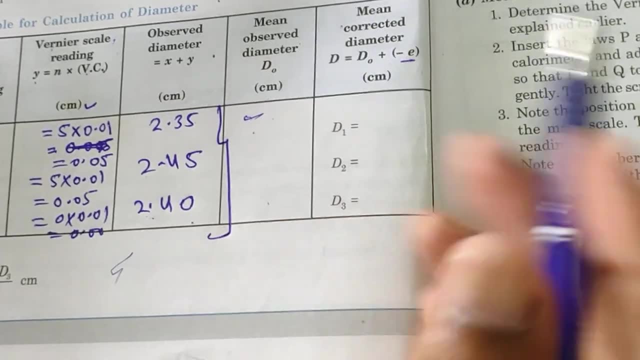 now you have three reading so you can take the diameter, mean diameter of all three readings. okay, now if we have some error, so we can plus minus the error. If there is are negative error, so we can add them, and if there are positive error we can. 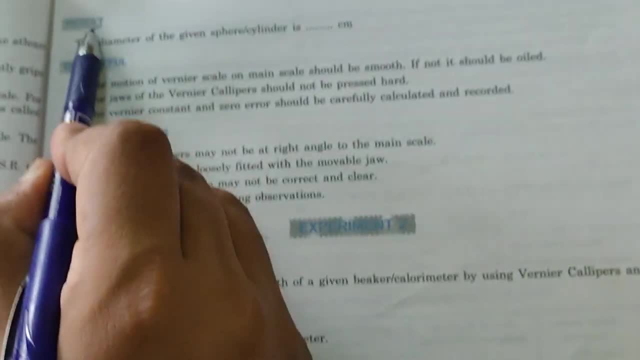 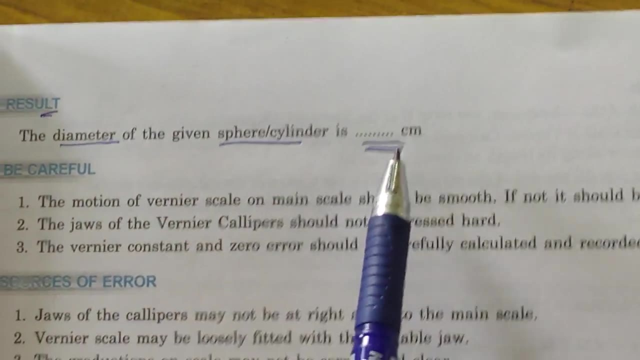 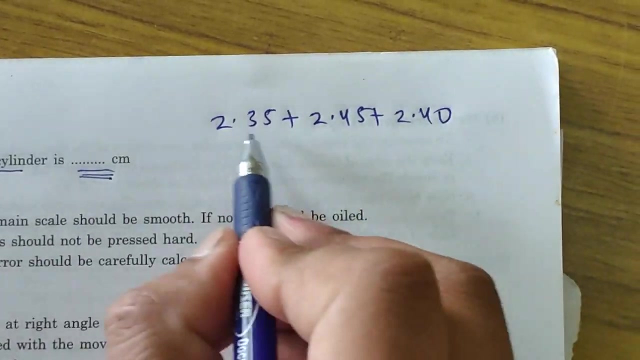 subtract them. okay. so after the calculation we have the result: the mean diameter of given spherical cylinder in up to two decimal in centimeter. okay, we can calculate this: two point three, five plus two point four, five and plus two point four zero, and divide by three. okay, so you can calculate this diameter and this is your result. okay. 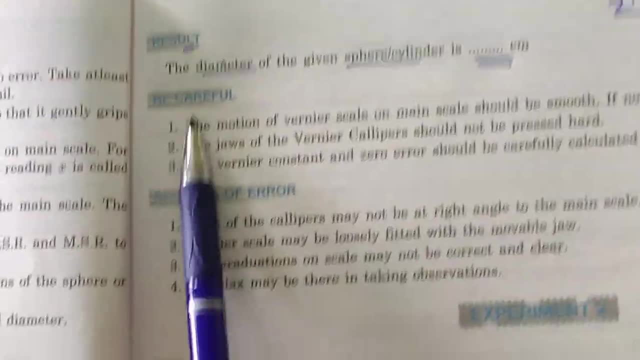 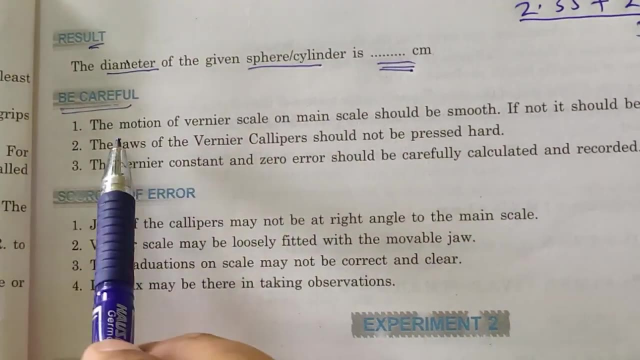 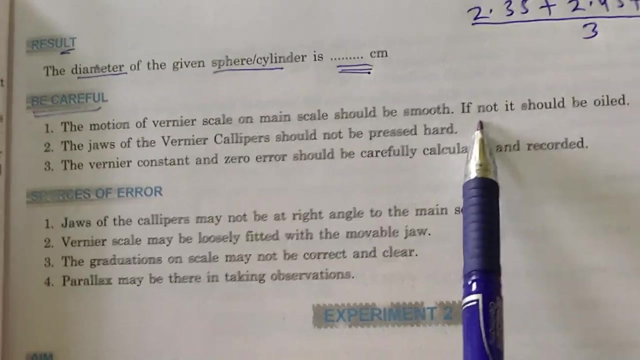 Thank you. So what are the precautions that you have to intake when doing the practical with the one year calipers? first, see the motion of one year scale on main scale should be very smooth, okay. if not, you should be oiled it. second thing, the jaws of one year calipers.